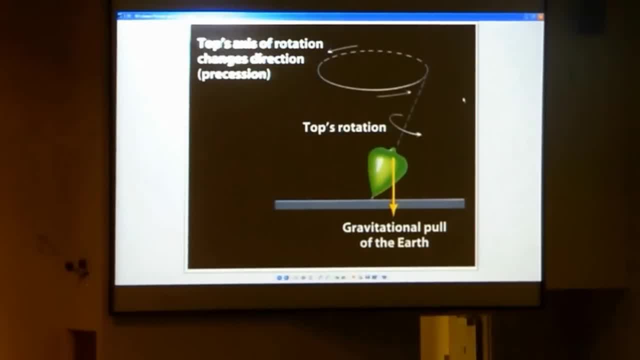 This happens if you have a body that's not perfectly spherical. If it's perfectly spherical, it won't do this, But if it's not perfectly spherical and there are forces tugging on it, it will not just stay in the same direction. So if this is in space, far away from any 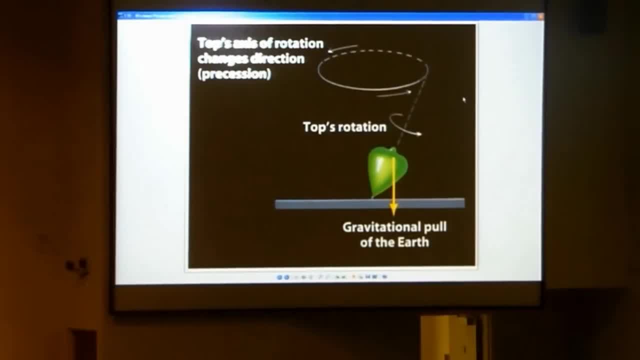 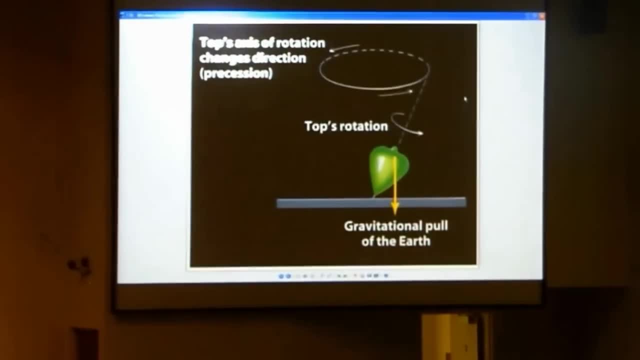 massive body. there are no forces. If you spin it, it'll just keep spinning. the rotation stay the same forever and ever, but there's a force tugging on it. the rotation axis will change as long as it's not spherical, and so the top is a great example of that. that's clearly not a sphere. there's. 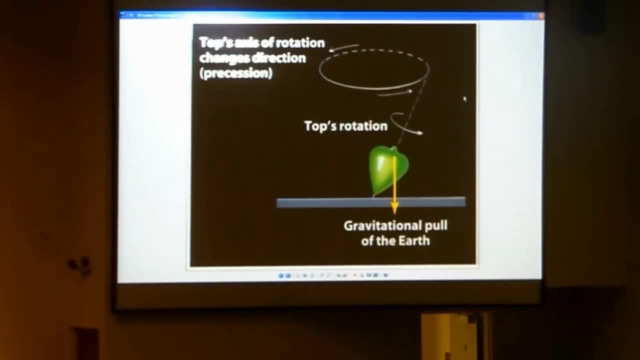 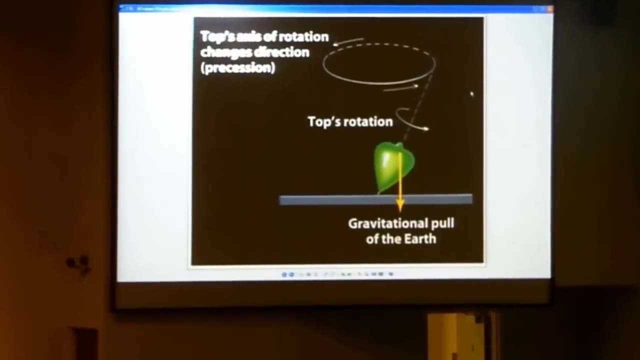 more mass distributed in some places than other places. so as you spin it quickly, it will process slowly compared to the speed of its rotation. yeah, i'll demo this right now. i brought a top. i brought a fancy top, so let's see if i can break this now. i've 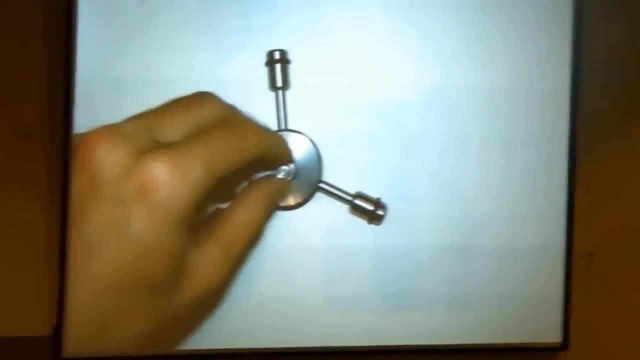 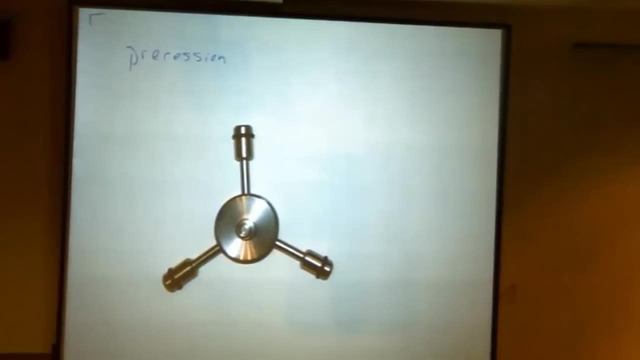 not just broken. okay, so this is the top. i can speed it up with this gizmo here. you'll all see it from the top of the top. i don't know if that would be useful or not, but that's how the the dot cam works. 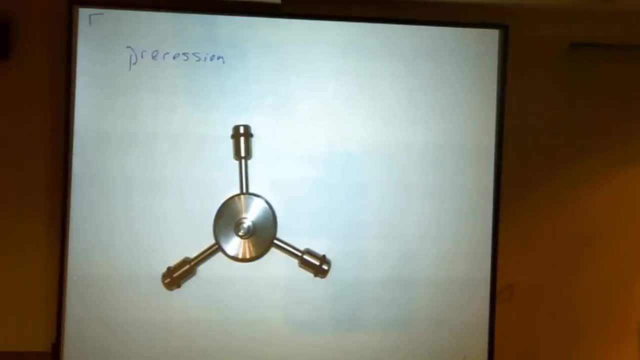 i also have a little movie of it from the side that i'll bring up in just a second. okay, this is what i used to spin it up, so i'm going to put it on the stand. here we go. okay, now i'm going to put it on the stand. hopefully i won't drop it. 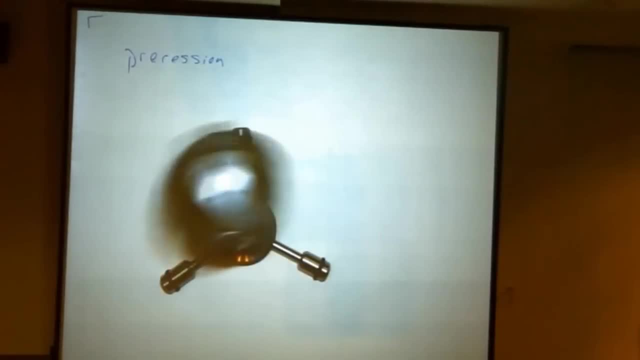 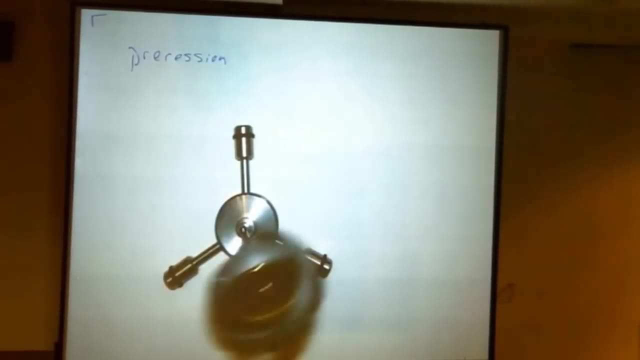 okay. so i mean it's a top view. maybe that's not the best view, but it's spinning super super fast. the gold in the middle is spinning super, super fast. then this is perceptive and you can see we got quite a degree of tip going on here. 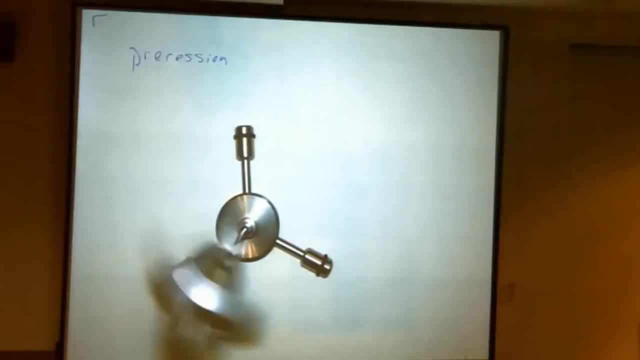 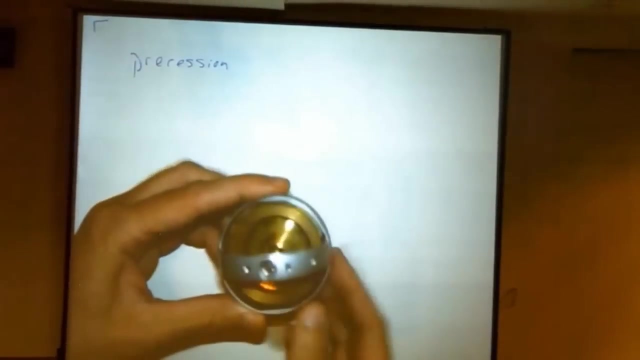 it's like a hundred dollar thing. i don't know why they let me take it and use it. this is going to end badly in just a second. okay, there we go. i'll show you a movie of it from the side, but, and the idea is, this is not a perfectly spherical distribution, looks like it's here. 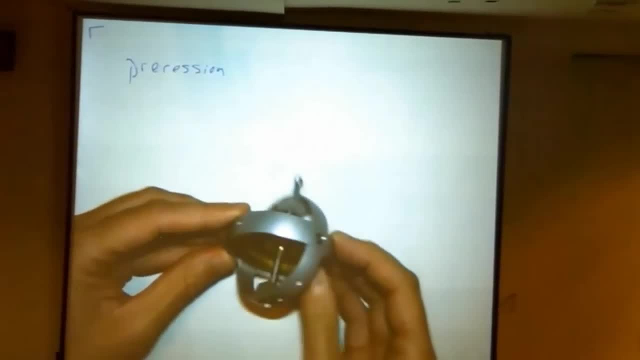 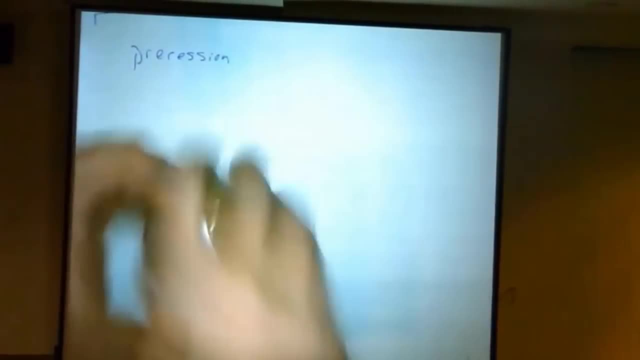 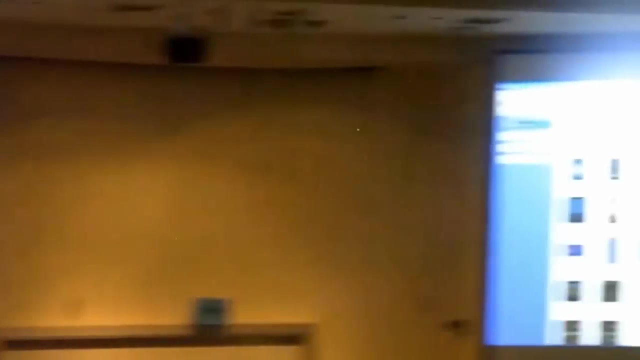 from this axis, but here it's clearly not sphere. the mass is kind of in the middle and this uh disk like structure here, because this was spinning very fast there and then it's processing on top of it. let's see, i got the movie, this movie of the exact same model. some reason movies take off. 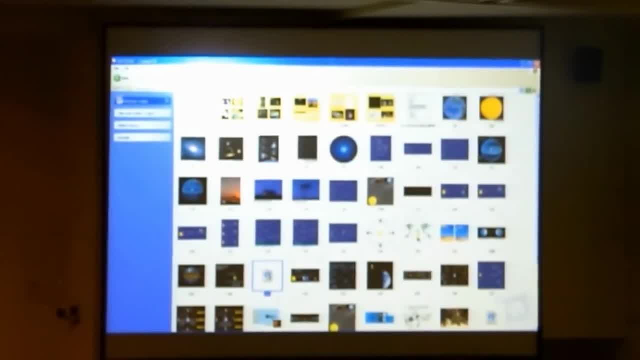 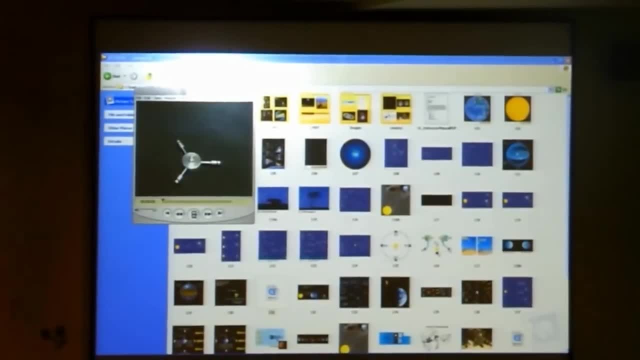 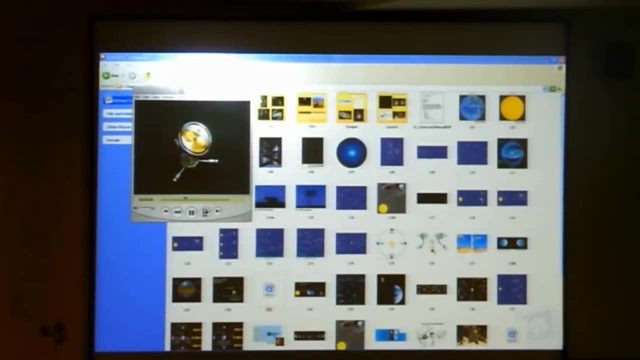 a lot of load on my laptop. it'll come off, though one of these days. it's not neat, okay? so again, the gold thing is spinning so fast you can't even see it, but it's processing as it goes, and just because it's not a spherical distribution. 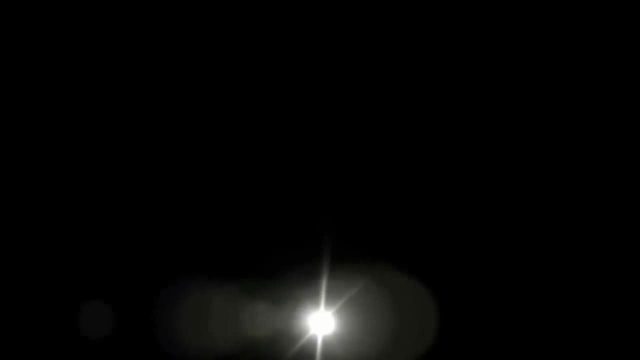 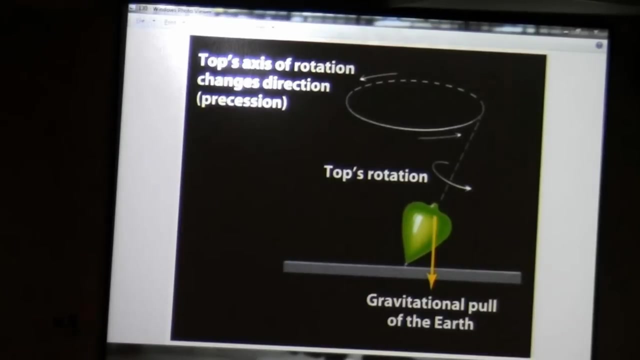 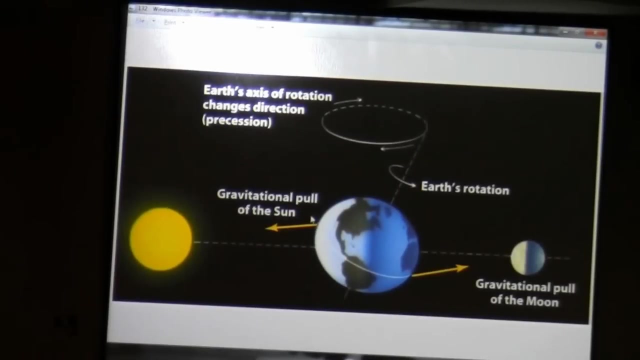 in a force, the force of gravity, is pulling you in one direction. so that's precession with the top. the question is: does the earth system qualify? but does the earth system qualify? and at first you may say no, earth is a sphere and for something to process it has to be aspherical. earth, it turns out, isn't perfectly. 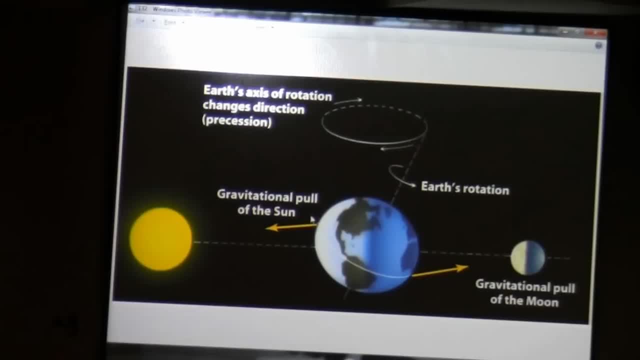 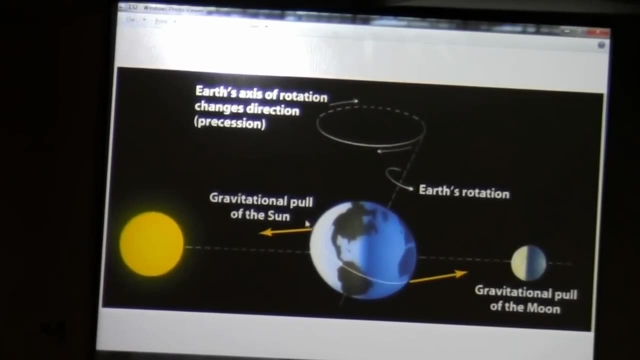 spherical, very, very close to spherical, but it's not perfectly spherical. it's because it's rotating very quickly. any object that's a little bit flexible, if you spin it really quickly it becomes oblate. i've never really developed a good demo for this, but i'll just draw the basic idea. 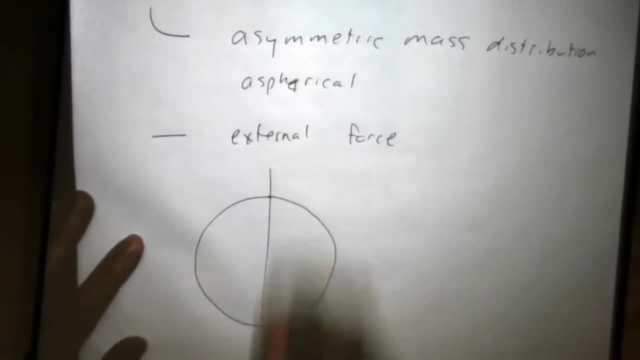 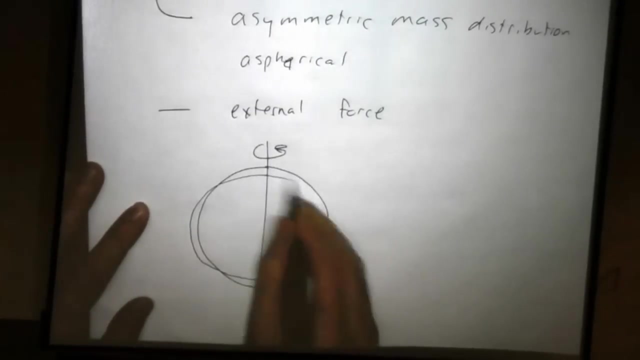 basic idea. here You start with the spherical distribution, and if it's spinning it becomes a little bit oblate, which means a little thick around the middle. here The mass distribution of Earth changes because of the spin. You can kind of get the idea if you're in a car. 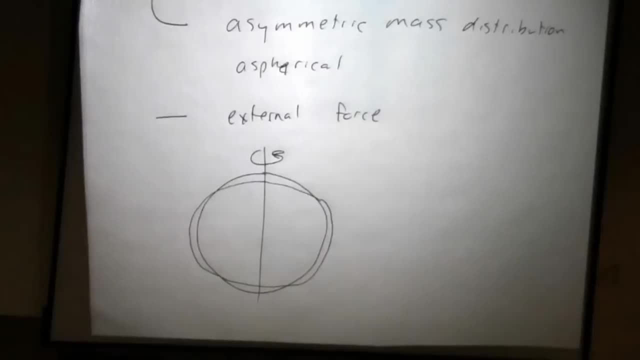 and you go around a curve very quickly, you're kind of thrown to the outside. Or if you're racing around a track, you feel that force pushing you to the outside. That's what's going on around the belly of the Earth. The Earth is spinning, It wants to fly out And 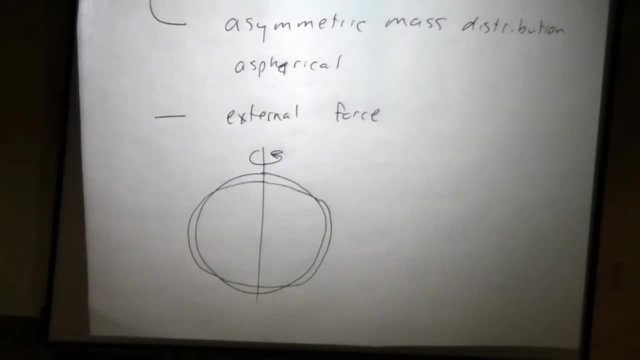 so the mass distribution changes a little bit. Not this much. It's a very, very small amount. You can't see it with the naked eye. It's stronger with the gas giants like Jupiter and Saturn. In the case of Saturn, you get 10% oblation. It's 10% bigger across the middle. 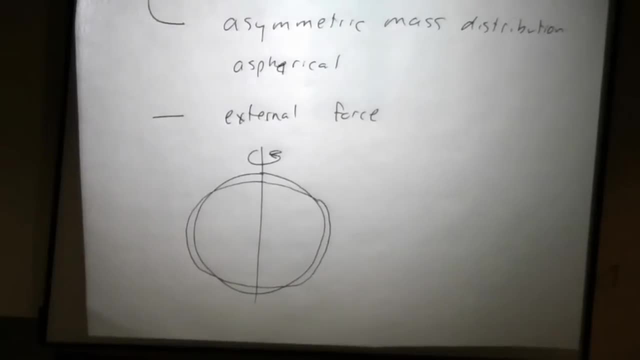 than from top to bottom. But that's because it's a big ball of gas, and gas is a little bit more flexible than the Earth, which is rock and metal. But you can measure it in the Earth. The Earth is bigger if you measure it this way instead of this way: pole to pole. So 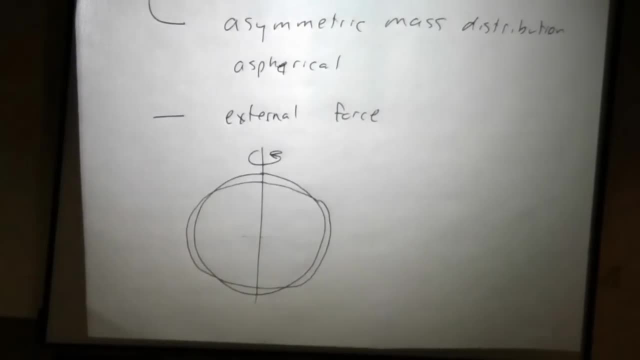 it's not a sphere. It's very close but it's not, And so it can precess. Since it's close to being a sphere, it can't precess very quickly. You can have very slow precession Now the other thing you need is an external force acting on it. In the case of the Earth, you have two external forces. in the plane of the solar system, pretty much, You have the Moon tugging on it and farther away, you have the Sun tugging on it as well. So we have these. 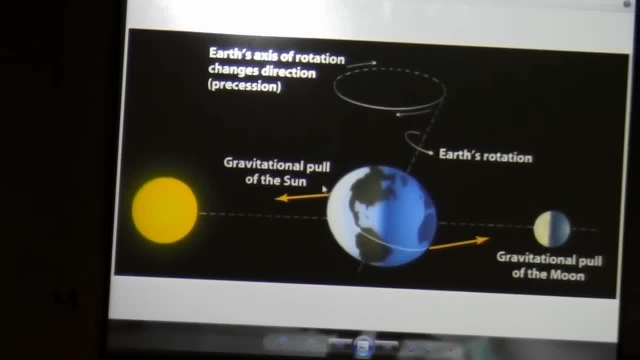 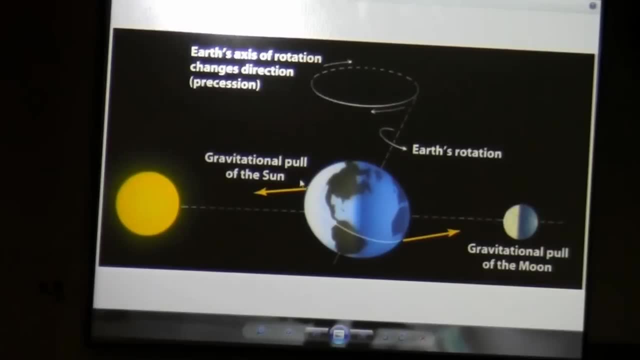 forces slightly different directions, Not down because there's no giant force of gravity like on the top we saw previously, but in the same plane as it, And so you do get very, very slow. precession: It rotates on its axis once a day. It precesses once every 26,000 years. Very slow motion compared. 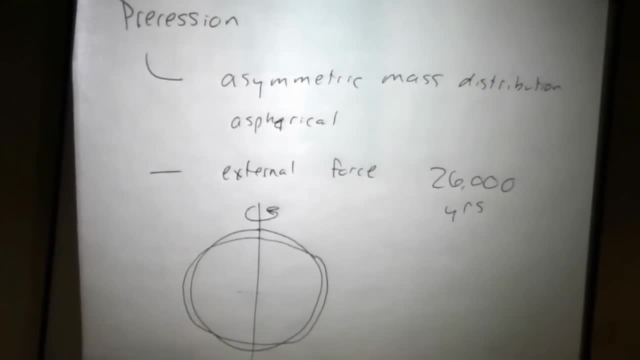 to the rotation 26,000 years. So what does that mean? Well, we've got the globe here and over one year it goes around the Sun and tilts. It doesn't change that much, But it's a very, very slow process. 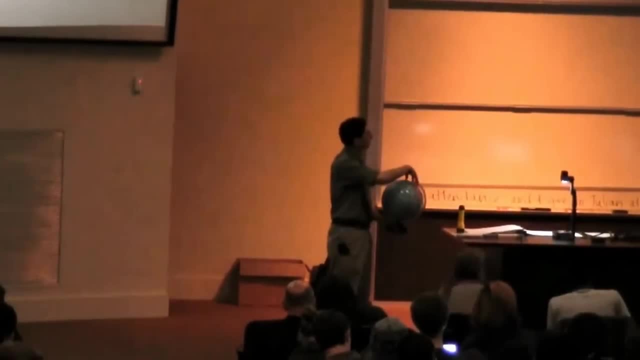 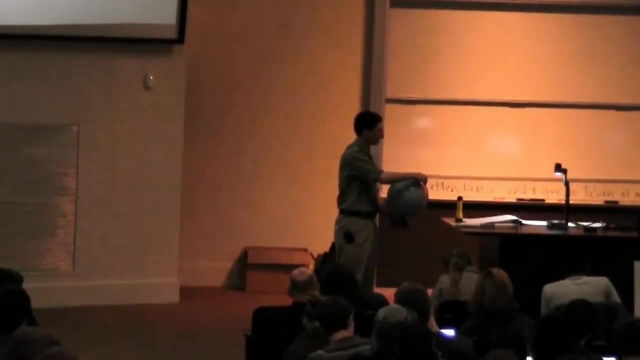 It doesn't change that much, But over time it will, And let's see the precession's in the opposite direction. So all the motions we've been talking about are counterclockwise. Precession is clockwise, So it's going to precess like this: The tilt's going to move. 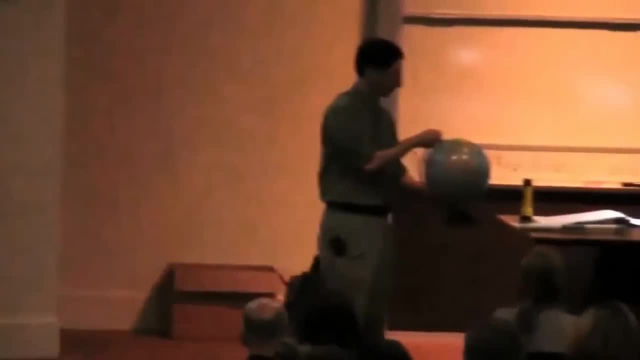 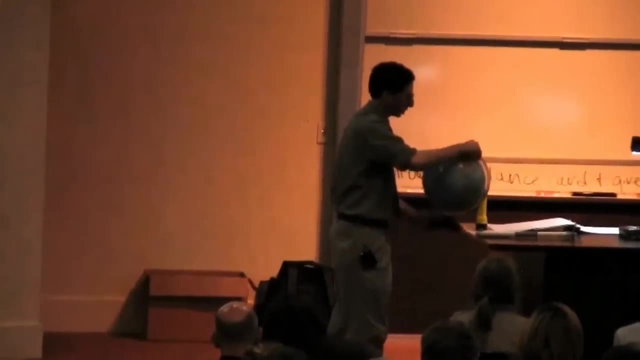 like this: After 13,000 years at this configuration in the orbit, it will now be winter instead of summer. So we start with summer and we go around, come back summer, go around, come back summer. But over the years we're going to precess just a little bit, And so summer's. 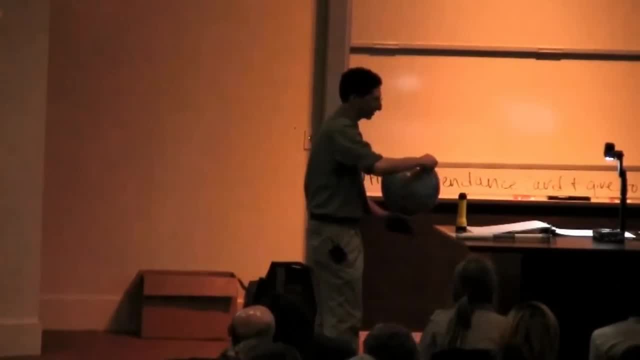 going to come just a little bit earlier And the next time we come around it precesses a little bit more. Summer's going to be a little bit earlier And it's a small amount. You don't notice it. year to year It's 20. minutes every year. The seasons start 20 minutes earlier than you would expect from its position in the orbit, So it's not like our calendar flips. Our calendar takes this into account. Check the time: Got a few minutes. Our calendar takes this into account. So summer will always. 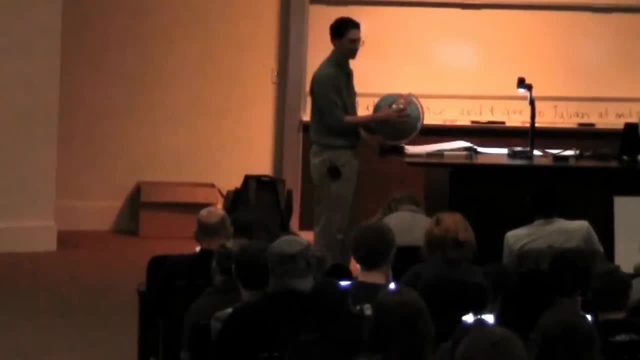 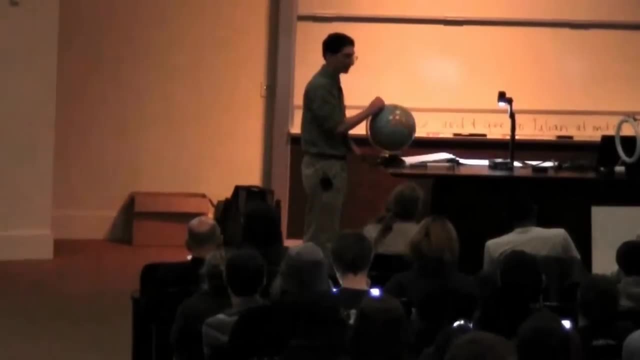 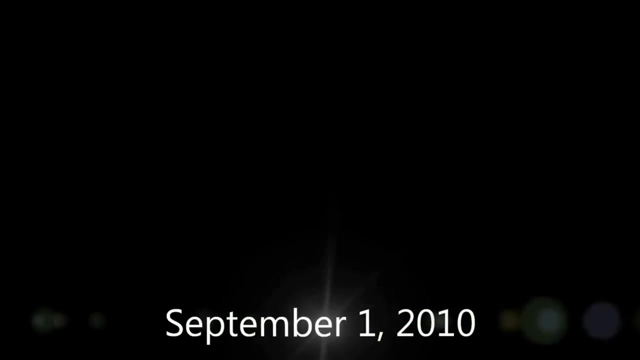 start on June 21.. But in terms of the position on the orbit, the seasons do come a little bit early. So after 13,000 years, what was summer over here is now winter over here, And then what was winter is summer another 13,000 years from now. The pole star changes, which makes sense. The pole star Polaris is the star that just happens to be in the direction of the rotation axis of the Earth. If I change the rotation axis of the Earth, I'm changing the star, or whatever star might be in the direction. 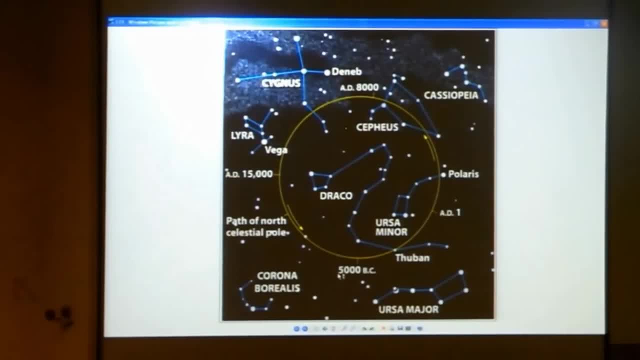 of the rotation axis of the Earth. I'm changing the star, or whatever star might be, in the direction of the rotation axis of the Earth, But Polaris will not be directly above. So this circle here corresponds to where the rotation axis points at different times, Right, 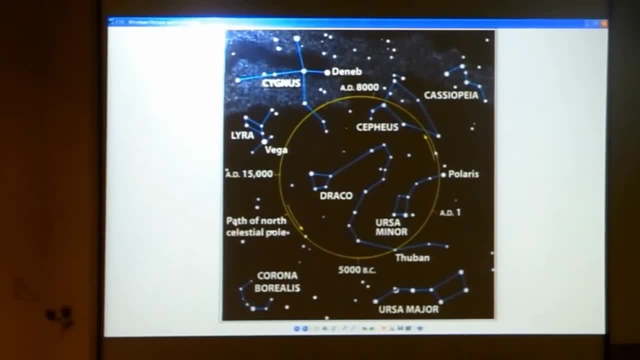 now we're kind of here close to Polaris. As the rotation axis changes, we go forward in time and Polaris won't be the pole star. It would move farther and farther away. Eventually we come aroundI'm not sure what star that is, but that will be pretty close All of 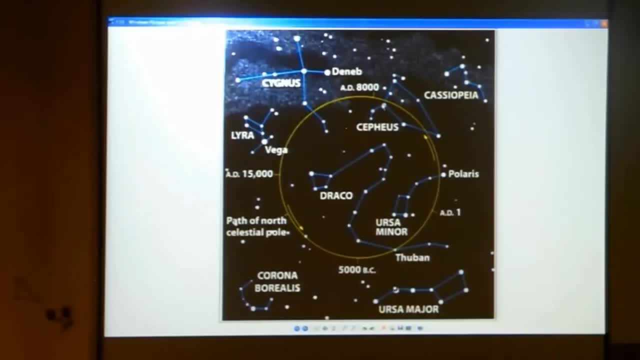 thesethis would be the pole star for a while, and then this one and this one. None of them are exactly there, and we shouldn't have it even until 12-13-18-18. Next week. exactly there You come over here. about maybe 12,000 years from now, Vega, or about 14,000 years ago. Vega is one of the bright stars in the sky. It's not super close, but it's so bright your eye will be drawn to it as a pole star. 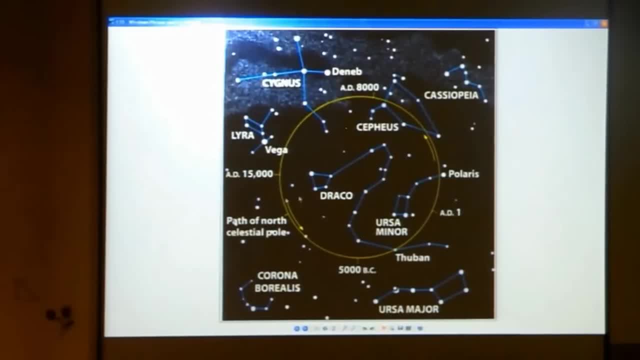 And you keep going forward in time or backwards. I guess they have to cycle the numbers at some point. But here's 5,000 BC, Maybe about 3,000 BC. you have Thubian, which is directly on the rotation axis of the. Earth. at that point in time It's not the brightest star in the world, but back then we didn't have light pollution. It would be easier to see, Maybe about as easy it is to see Polaris nowadays. So that was a true pole star, a north. 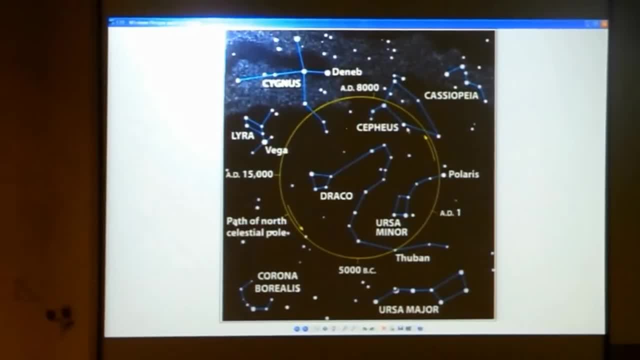 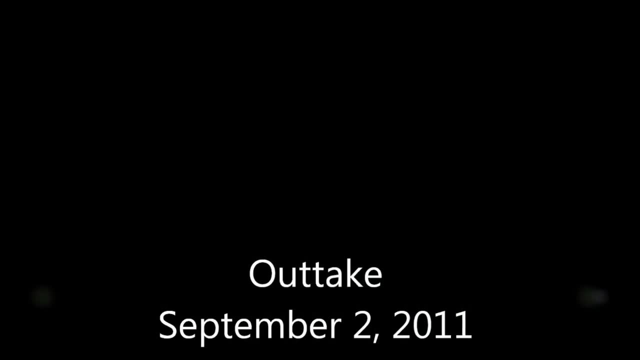 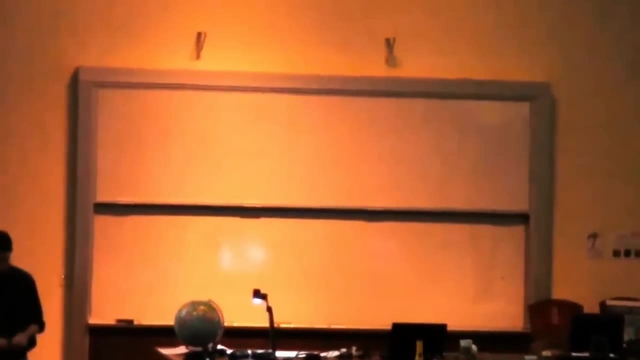 star And after 26,000 years you're back to where you started. Now. I used to have a really nice top. I stole it from the physicists and I was keeping my office, and then someone borrowed it back. Maybe I felt bad and gave it. 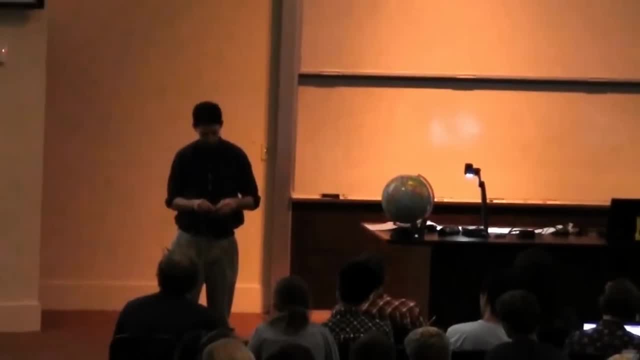 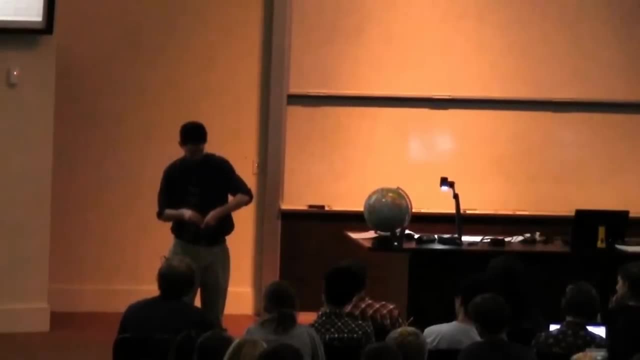 back. They either lost it or they hid it from me. I haven't figured out which yet, But they gave me this really crappy top and it's compensation here. So my other one was electric. Now I could just add a little motor and it was. 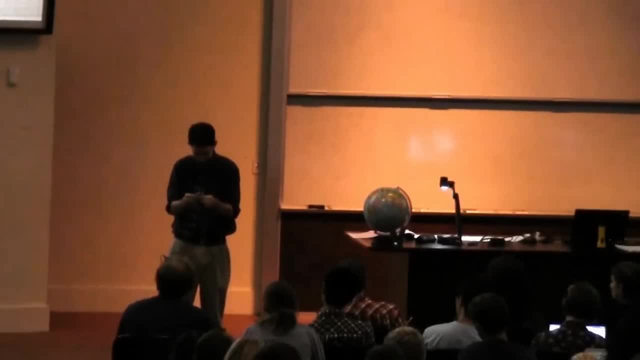 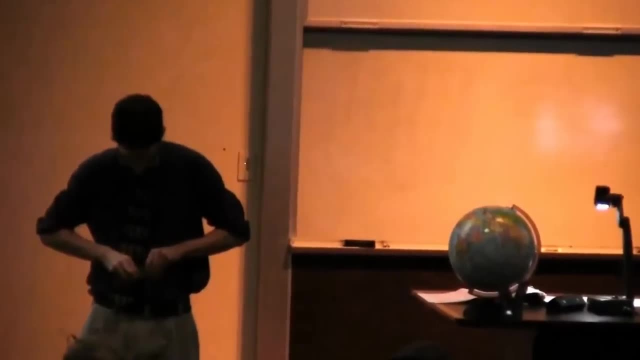 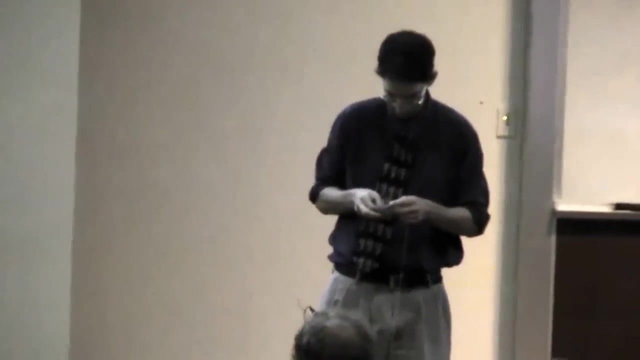 spinning real fast This thing. I've got to wind up with a piece of string and it's pain to do. Be patient, I'll get it. I did pre-wind it for the other section, but then I used it and didn't have time to set it up. 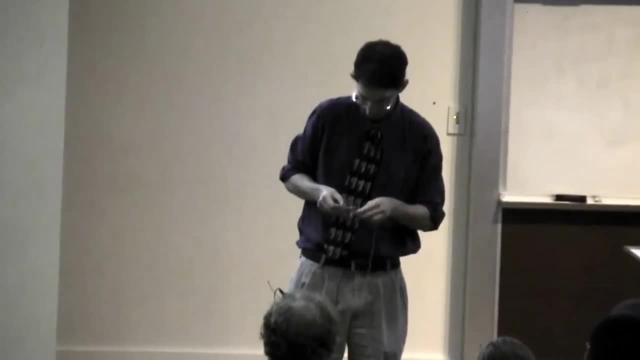 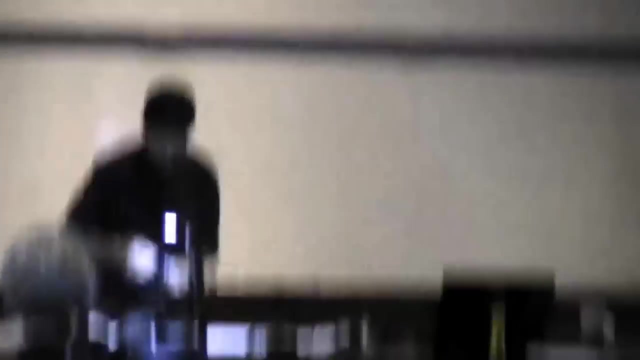 again. I'm getting it here. It'll be worth it, trust me. Actually, I probably won't, but okay, So that's probably enough for me to get it spinning. Here's the base. I'm going to set it on this thing. 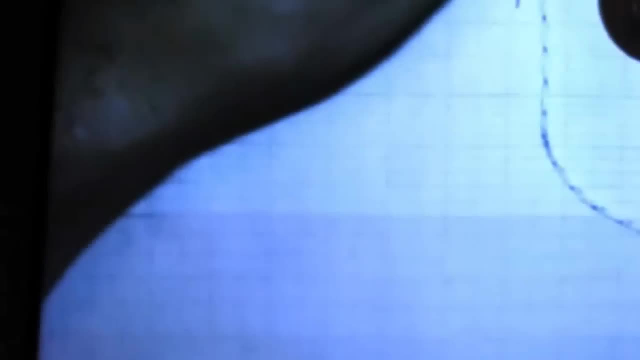 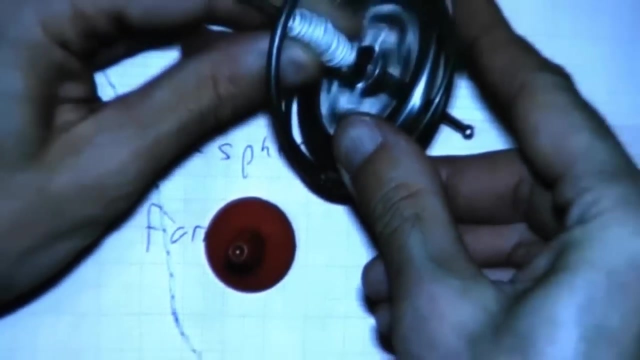 So, just so you see it before I spin it, We have this part in the middle here that spins And I've wound the string around. I'm going to yank the string really quick to get it spinning fast And I'm going to set it up on this And you have not the 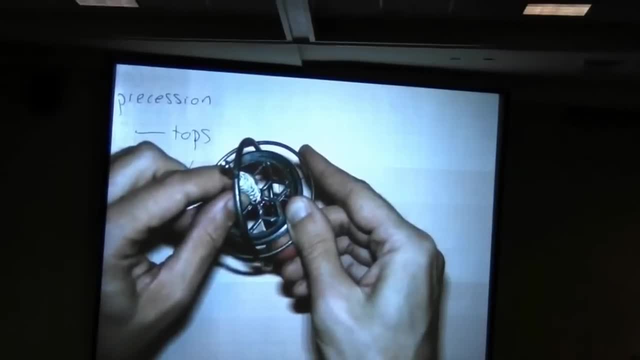 best view. You have a top view of the top. You'd be better to see it from the side, but you know it's too small and the classroom's too big. But after this is done, I'll show you a movie of my really nice 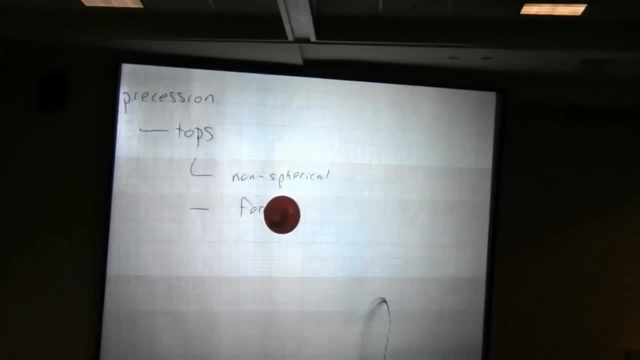 top that they're hiding from me. I know they are Okay, so I'm going to show you a movie of my really nice top that they're hiding from me. You know I have this lab with all these students. We build telescopes all over the earth and they don't. 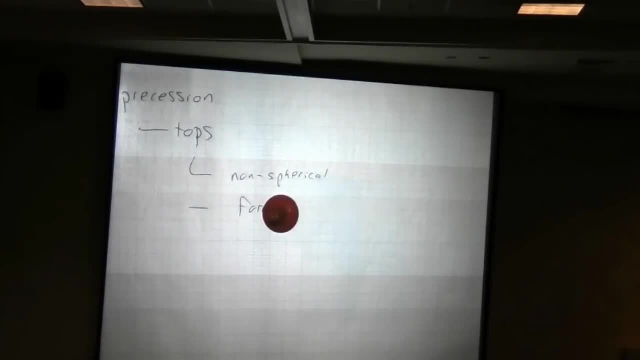 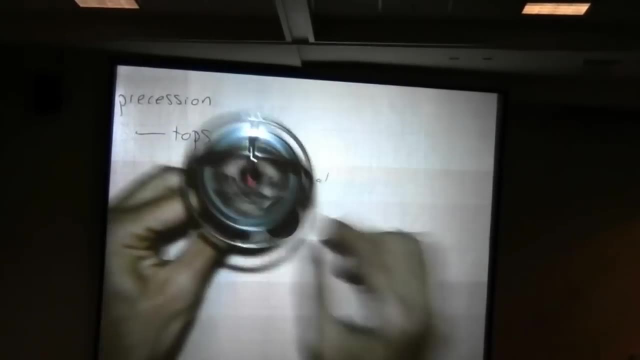 let me touch any of them. So I always break everything I touch, and that's probably going to be the case here, But let's see how it goes. Okay, it's spinning fast. Now I've got to somehow get it on here. 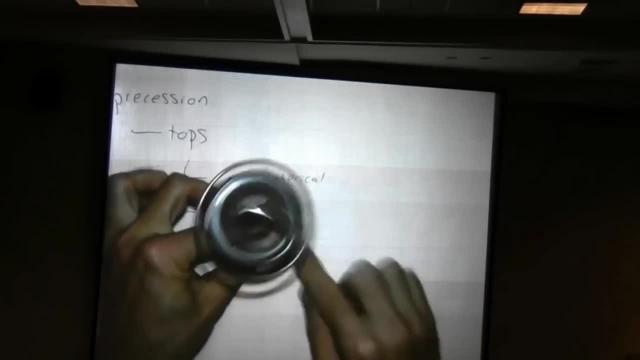 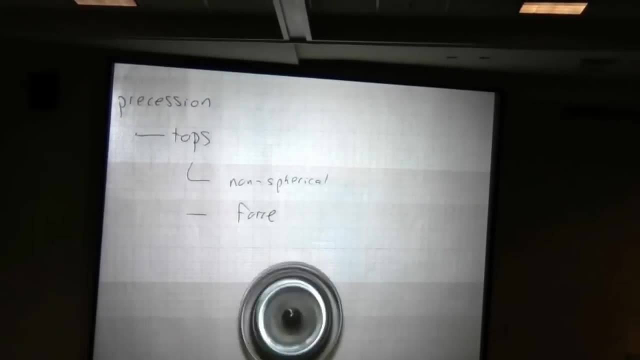 I think it's going to fall over, but there we go. Whoa, Damn it, It's going, though It's going. It's not sitting on the base, but you see it processing there. It's spinning really fast. It's processing slower than it's spinning. 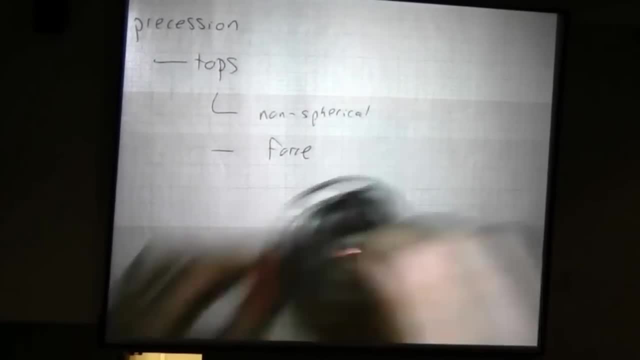 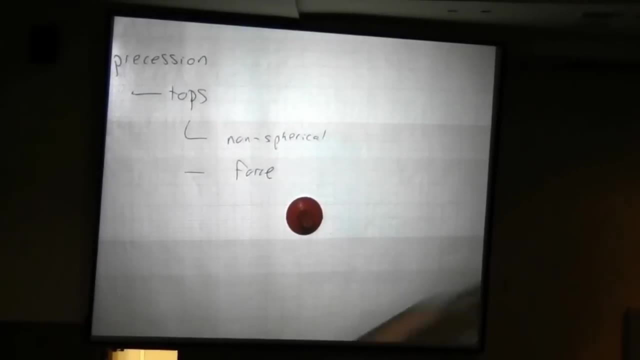 And now it's kind of straight up and down. Let me see if there's still any juice in it. No, I don't know. It's probably not worth me winding it up again. I don't know. Let's try it. Let's try it. 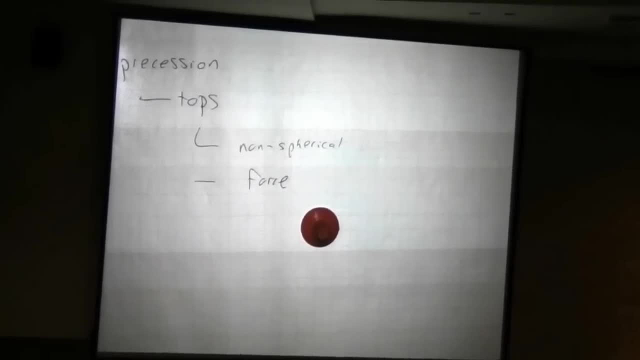 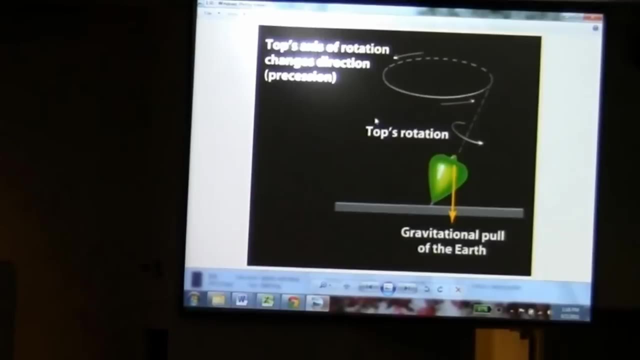 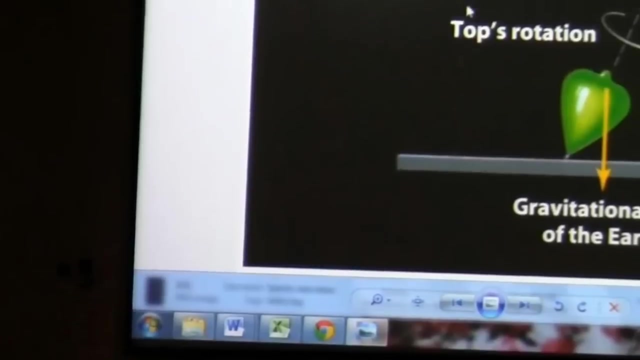 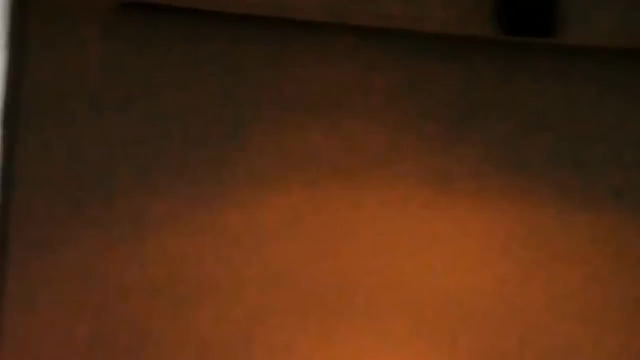 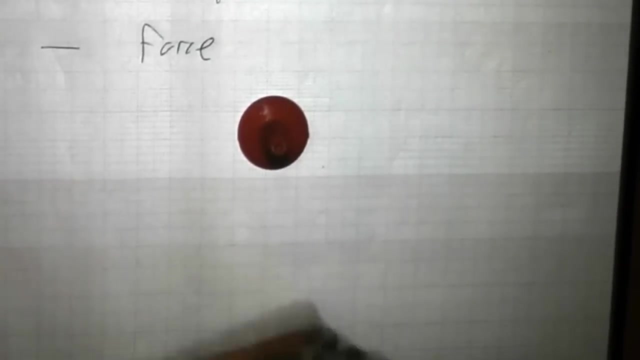 This is fun. I'm going to try it one more time. Damn those physicists taking the top. I stole from them. Okay, we're going now. Yeah, it's going faster. Okay, And I feel the thing wanting to process in my hand. 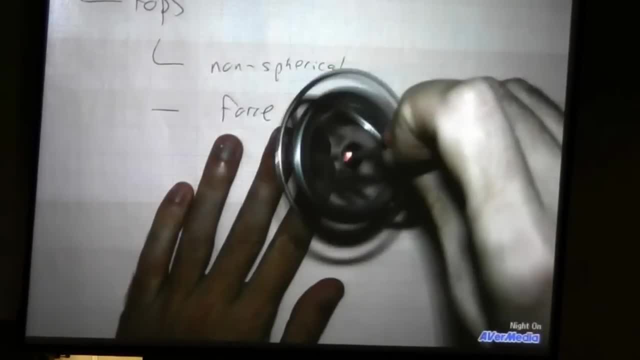 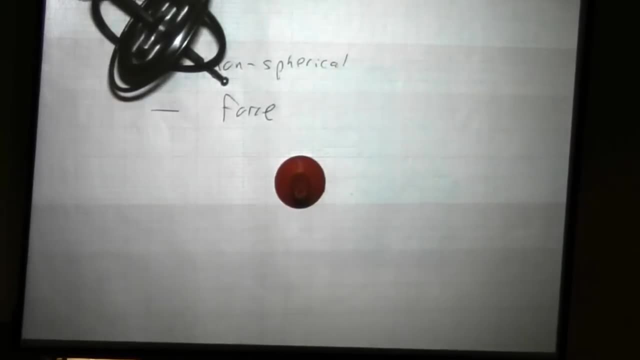 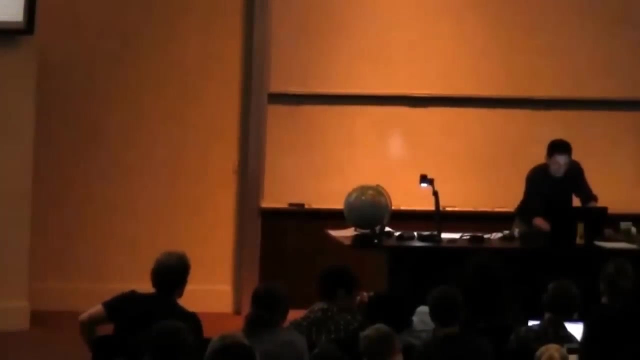 Get on there, damn it. Okay. Laughter What? Oh, fuck. A little bit less perception, Fuck it, Excellent. I should have done that in the class. I wasn't even videotaped.